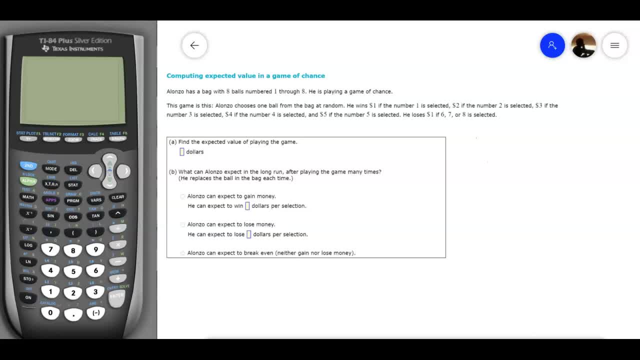 all right, so in this exercise, we're going to learn how to compute the expected value of a certain game or certain distribution. all right, so in order to calculate the expected value of any distribution, we need literally all the outcomes. so for this purpose, we need either the frequency distribution table or the probability distribution table. 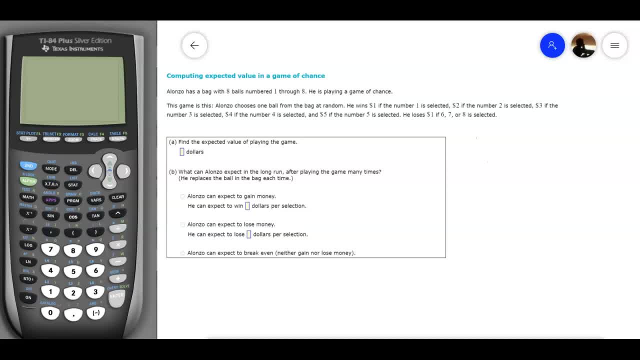 all right, before starting the calculation. so I'm gonna use the frequency distribution table because it's kind of easier for this problem and it's kind of simple. so I'm gonna start with the table here, all right? so in this table I'm gonna have the outcomes, so the x and 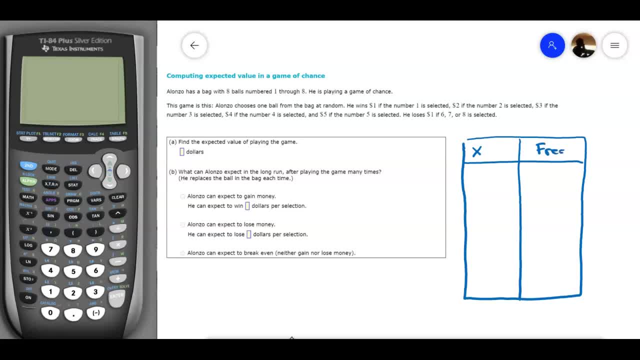 I'm going to explain to you the x and the frequency over here. right, so the X goes south when theector sausage strikes, первый line're going to be defined X's. actually, they are not the outcome in in the balls, right? so so, although the we 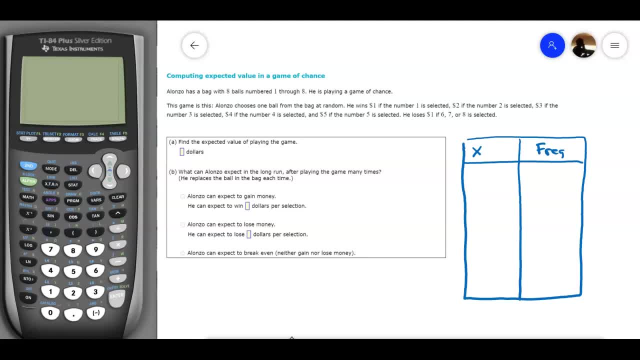 are extracting balls here, but every ball you can represented by a certain dollar amount, right? so that's what we're gonna focus on. alright, so we're gonna focus on the dollar amount and if you notice here that you're gonna be winning one dollar if I get to one selected, right, so there is a one dollar. so this is representing. 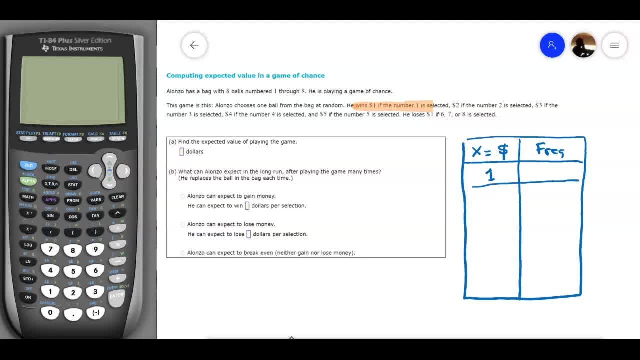 one dollar and the frequency of the one. it would be how many once you have, out of eight balls here, you have only one, all right, so that the frequency, and then we go to the second centers and you're gonna win two dollars if two is selected. so what does mean you are getting two, two dollars here if you are selecting. 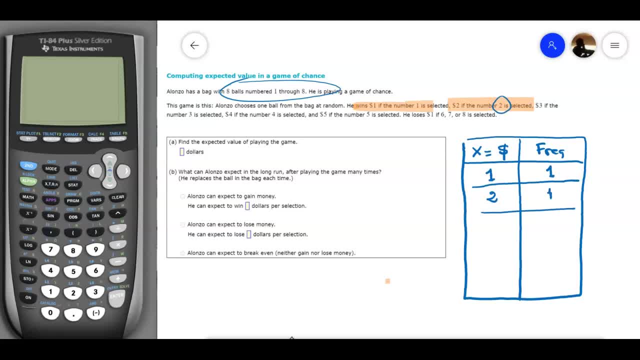 two, but again what? the frequency of two is only one. so you're gonna put one again and then you're gonna go to the next sentence. again, you're gonna get three dollars if you select three, so that's you can be. again, you're gonna get an amount of three dollars and the frequency of three, three out of. 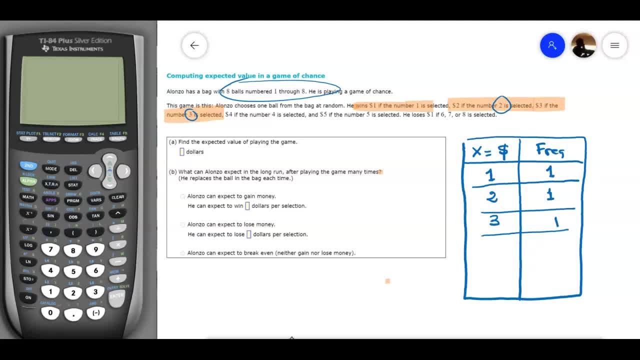 basically three, one, two, eight, so it's only one. three there. so frequency is one, and then again we keep going with the centers. you're gonna get four dollars if you select four. so the amount here is four dollars, all right, and the frequency here is one, because 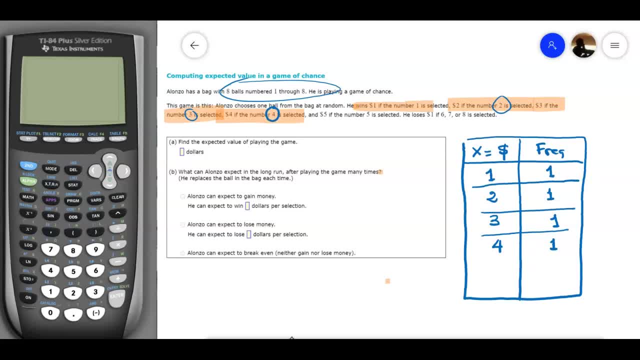 only one ball you can can get you four dollars. now we still have a five dollars as well, right? so we're gonna get five dollars if we select five. so maybe I'm so this: you're gonna be a five dollars and the frequency of five: again you there. 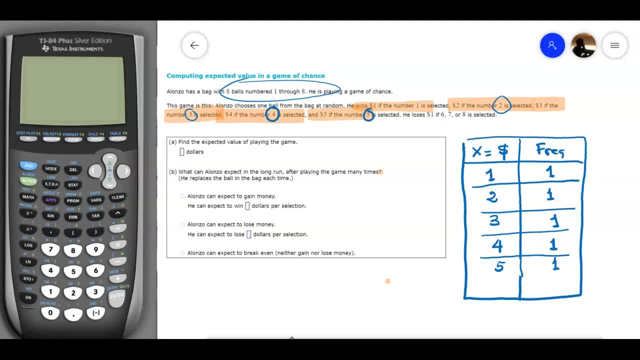 is only one, five, so you can be just one. now you're gonna lose one dollar. so the losing: whenever you gain, they are all positive, but if you lose you can be negative. one dollar if you get six, seven and eight. so the frequency here: who can make you lose a dollar? we are three out of eight. 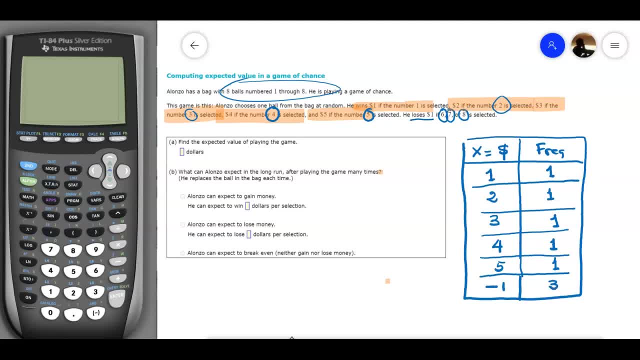 which is frequency of three. so here this you can be: frequency of three. so once I set up my distribution frequency table, I can go ahead to my calculator and plug in the numbers. all right, so you need to use the statistics and then you're gonna edit, you're gonna erase any table that you might have there. so in order to 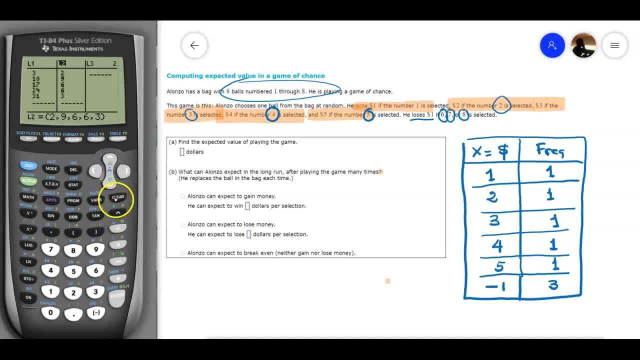 erase, you can go up clear enter and again you're gonna go up clear enter to clear the both columns, right. so now what I'm going to do, I'm gonna plug in the X's, which is one enter, two enter, three enter, four, enter, five, enter and then 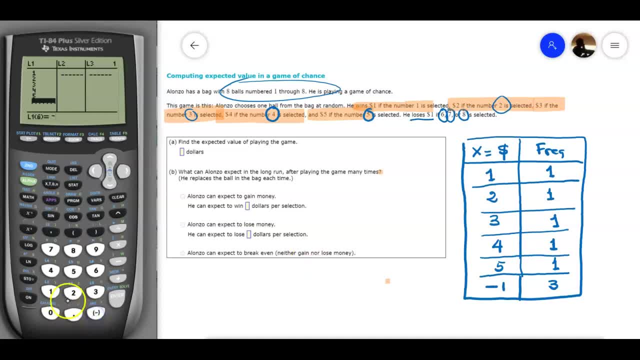 you're gonna be a negative one, so negative, I have to do this. negative and one and enter. so I plug in my X's. now I'm going to go to the second columns and I have to type in the corresponding number. so in front of one you're gonna be one, so you're. 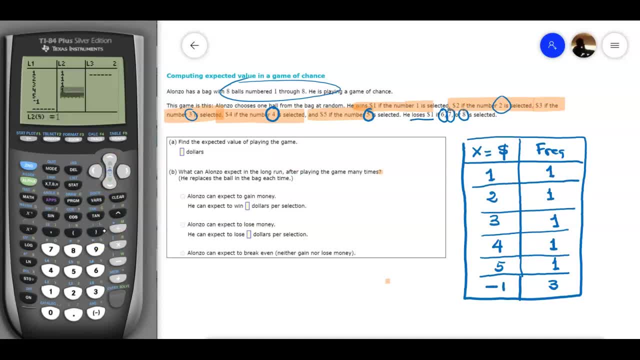